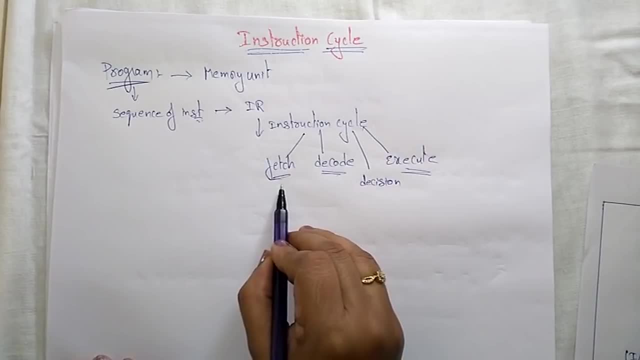 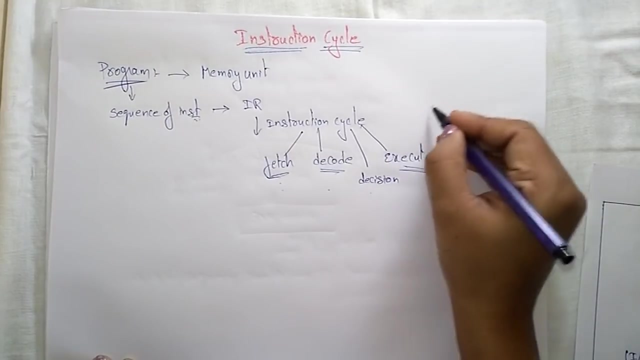 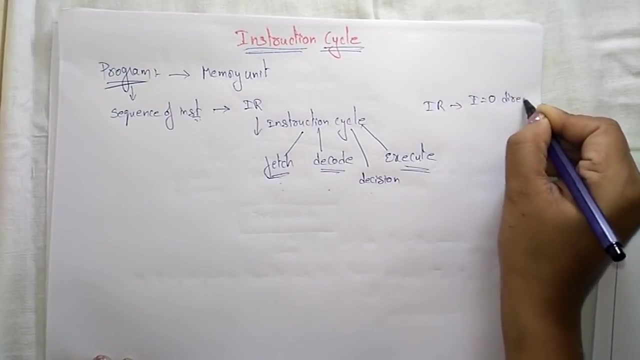 fetch is used to fetch the data from memory unit. after fetching the data that will be decoded in the decoded phase. after decoding, it reads the effective address from memory of instruction. if it is indirect address, suppose the instruction whatever it is present in the instruction register. if I is 0, it indicates direct addressing. we 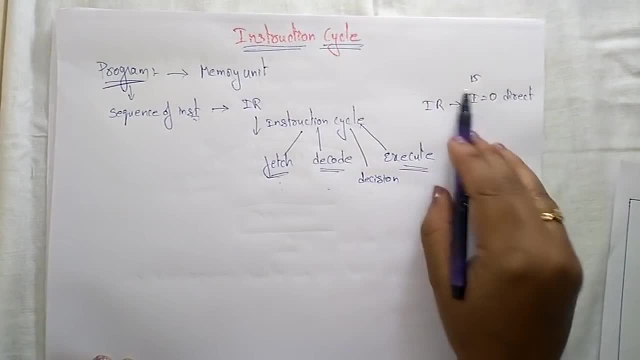 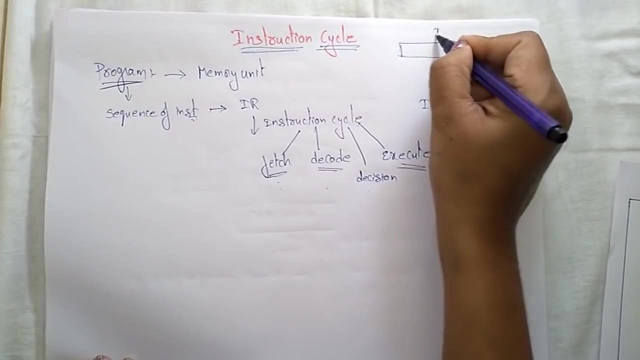 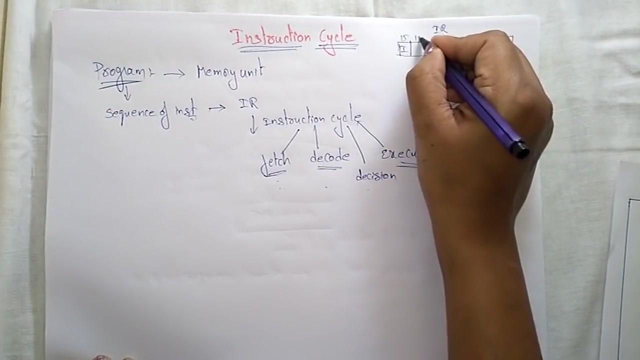 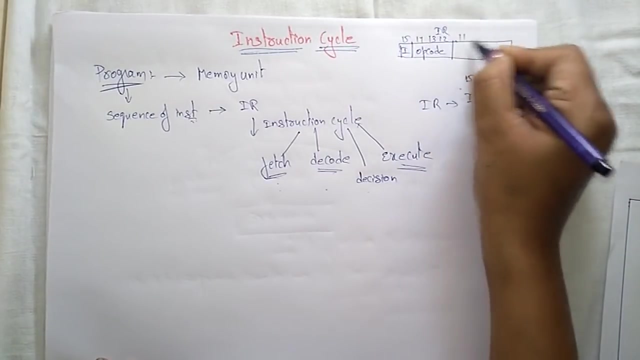 already discussed it. I is a 15th bit in the instruction register, so this is the instruction register. so this is the 15th bit. indicates that i and 14, 13, 12 indicates the opcode operation has to be performed from 11 to 0 is the holds the address. so this we already. 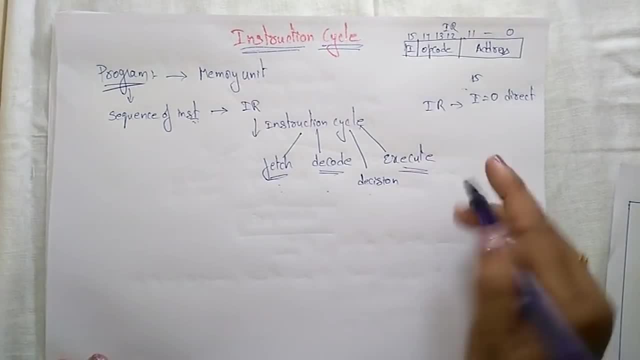 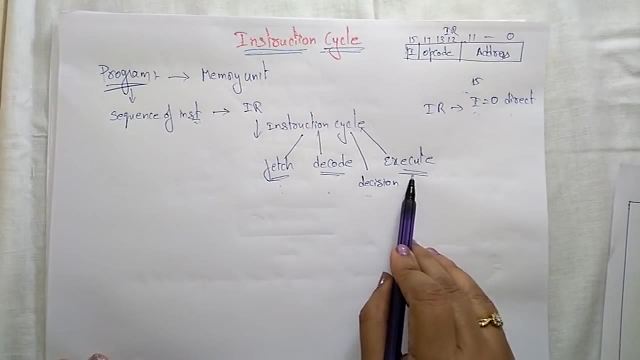 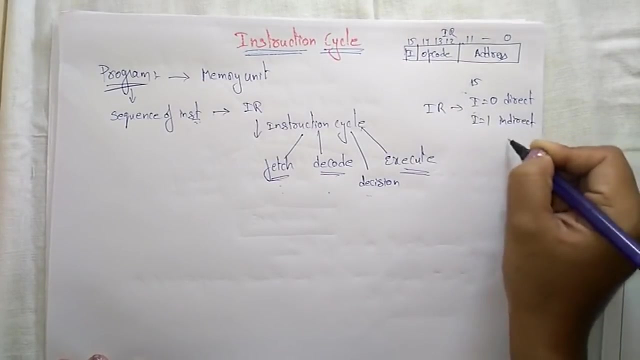 discussed in the previous slide. so here the I indicates: if it is 0, no need to go for the decision. it directly executes the instruction. if I is one means indirect addressing mode. so if it is I is one, then we have to read the effective address. effective address from memory of instruction. we have to 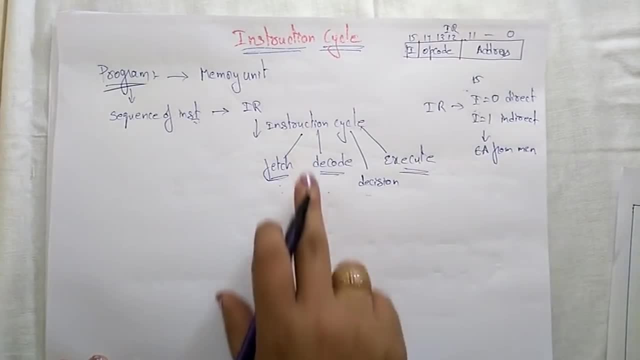 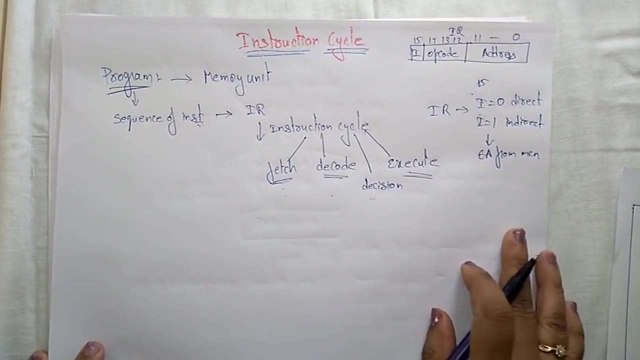 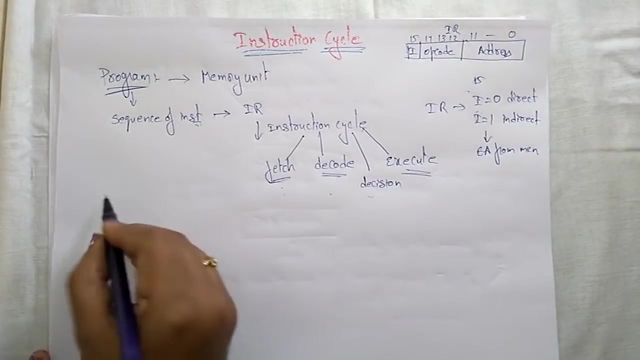 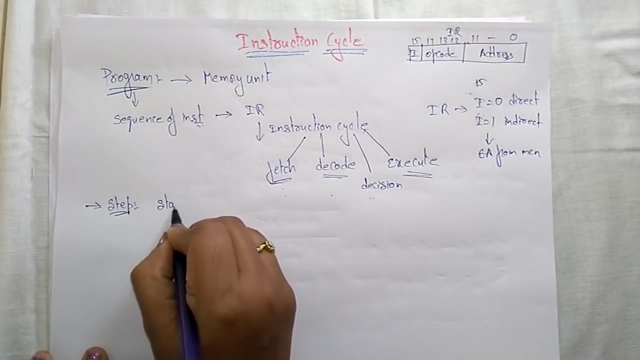 read the effective address from memory. so this is the instruction cycle. so let us see how the instruction cycle will be executed in the form of a flowchart. so before going to discuss the flowchart, let us see the steps that are coming in the flowchart. so first step is we have to start the program. so when? 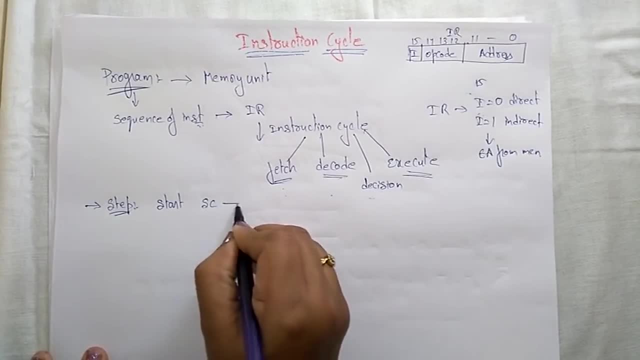 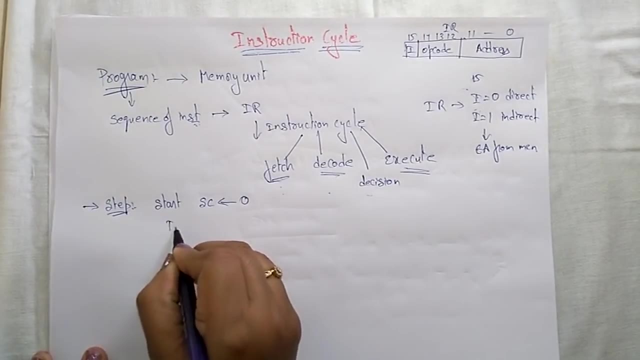 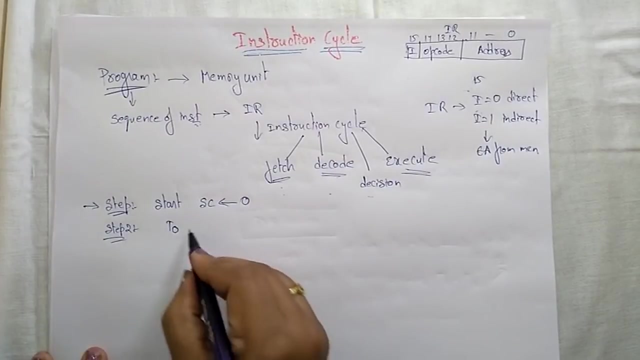 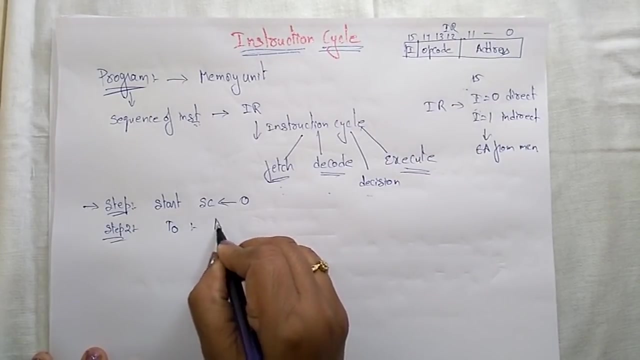 it this when we will start the program whenever the sequence counter will be 0. so sequence counter is 0 means the timing pulse starts from T naught. so at the time of T naught, step 2. so during time, during the timing sequence T naught, the program counter will be placed in the 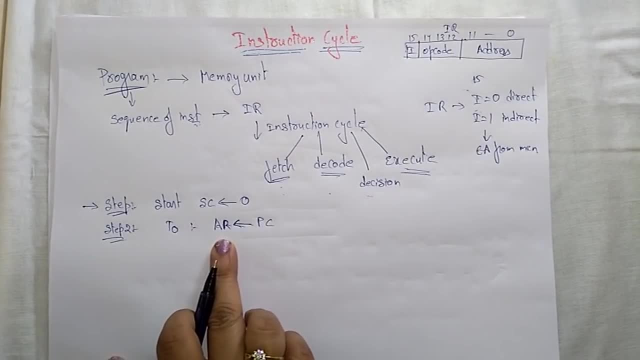 address register. so what address register contains? whatever the address that is present in the program counter that will be placed in the address register. program counter is nothing but the address of the next instruction to be executed. that will be stored in the program counter. so in the next step we 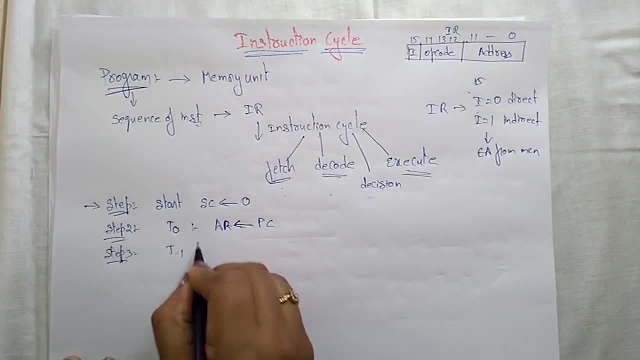 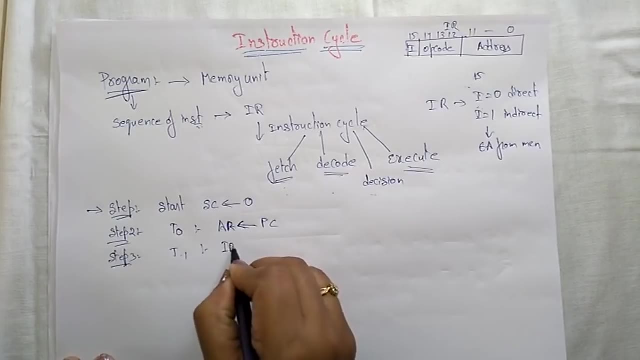 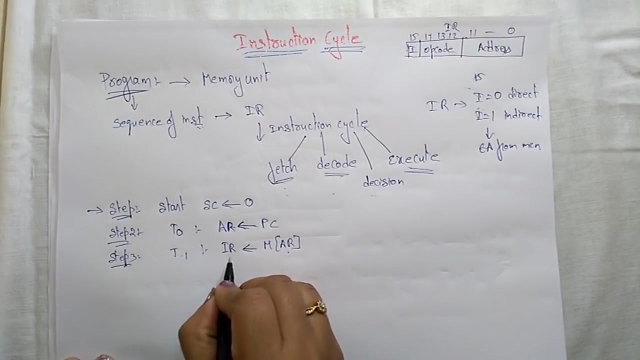 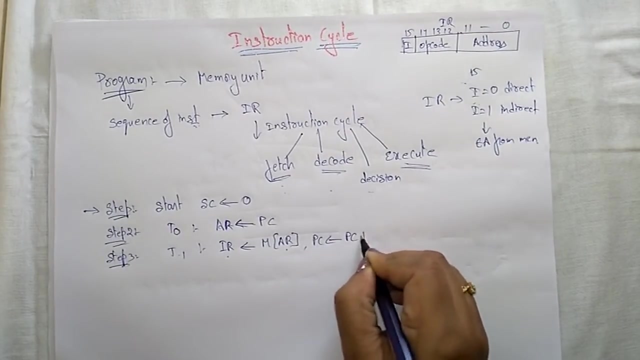 going to give data to the program for invokingored in the program and then we will compare the values of the recurrence value in the program again. let us solve the problem of the execution. again, counter will be incremented by 1 means the next instruction that has to be executed, that 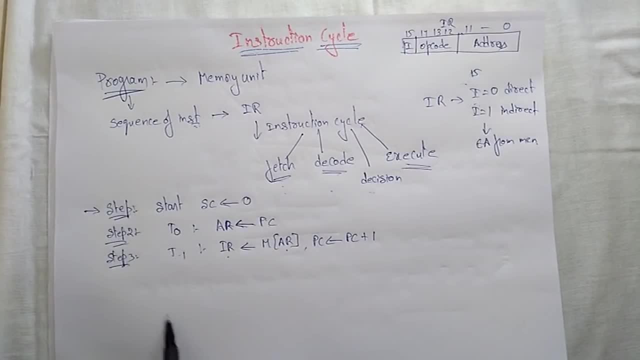 will be stored in program counter. so whenever the operation is over again it takes the instructions, which will be incremented by 1 in that location. that location will be transferred to address register and the content of that address, the operation that has to be performed, will be moved to the instruction register. so this everything will be done at timing signal t1. 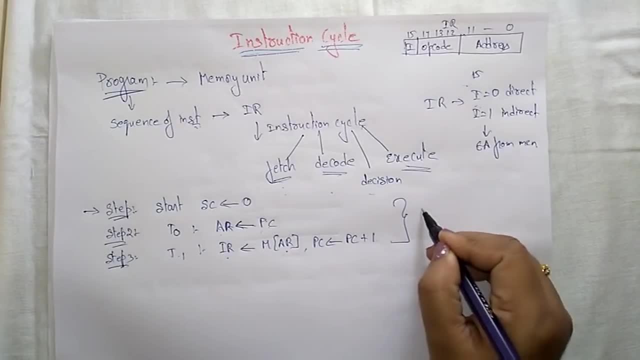 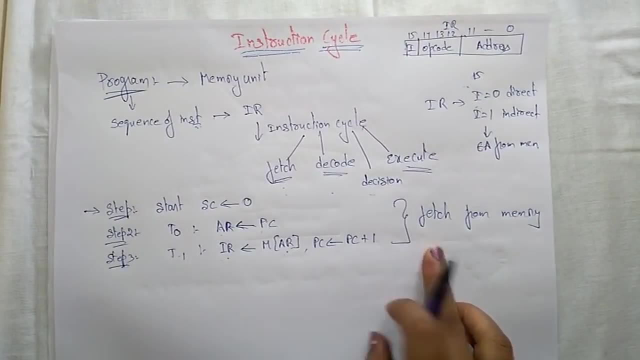 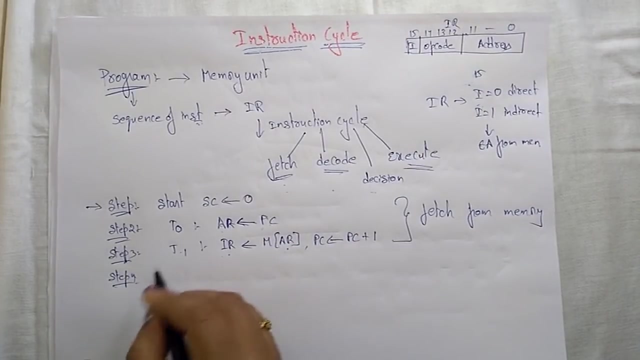 so this during t0 and t1, you, we are just fetching the data from memory. so this is the fetch cycle, so you are just fetching the data from memory. now coming to next step, step 4. so during t2, during the timing pulse: t2, uh, timing. 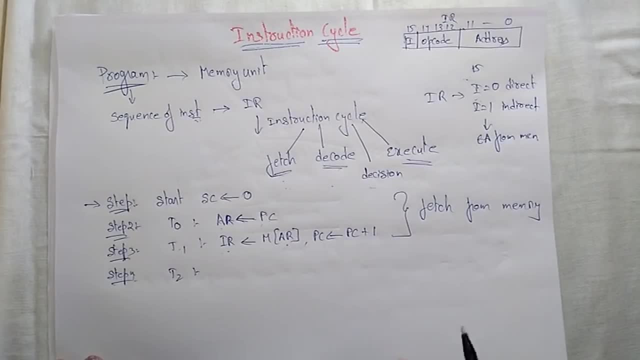 signal t1 and t2 will be done at timing signal t1. so this, everything will be done at timing signal t2. what, uh, the instruction will doing. so this is the after fetch. we have to decode the instruction, we have to convert whatever the instruction that we are fetching from memory. so decode first you. 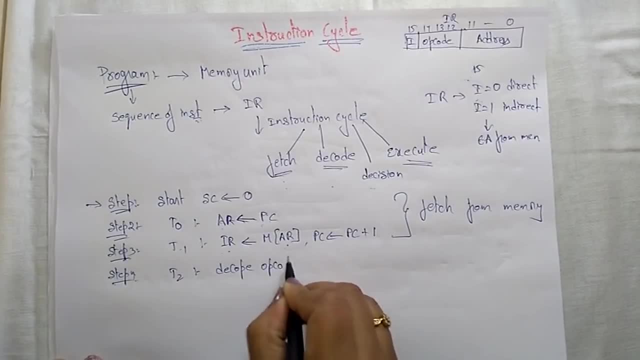 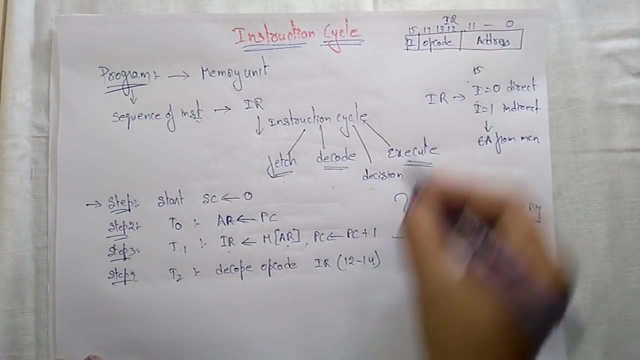 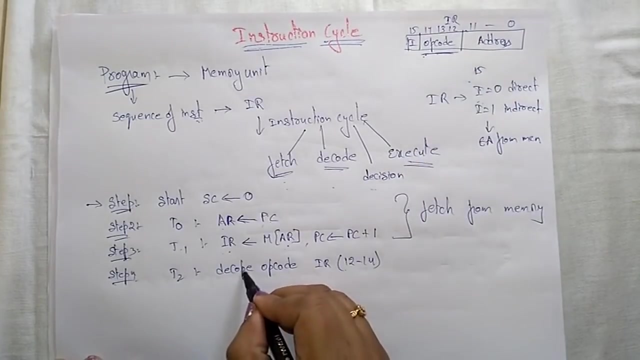 have to decode the opcode. so where will be? the opcode is present. the opcode is present in instruction register. so from 12 to 14 bits, the opcode will be there. so this is the opcode: 12 to 14 bits. so this will be decoded. decode: opcode in the instruction register. after that: 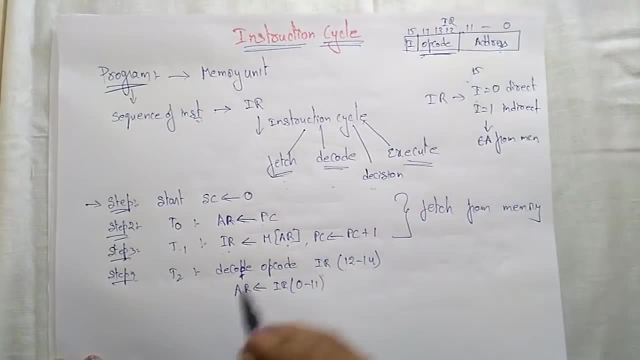 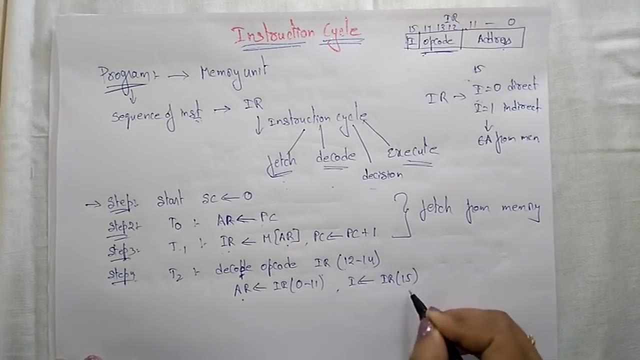 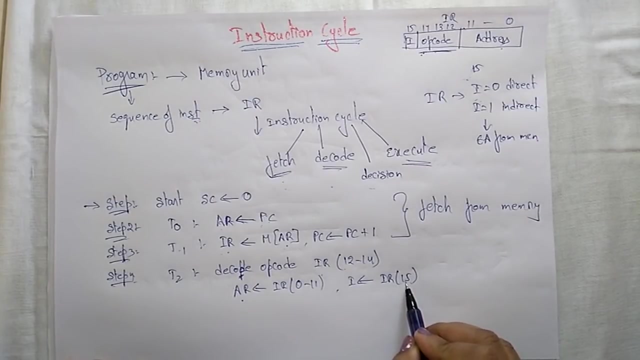 the 0 to 11 bits, which holds the address. that will be placed in the address register. then i indicates the 15th bit. whether it is 1 or 0, that will be decided based on the instruction that is given. so if it is 1, it is indirect 0. 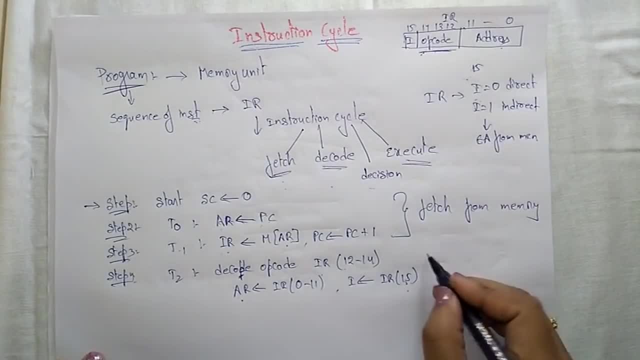 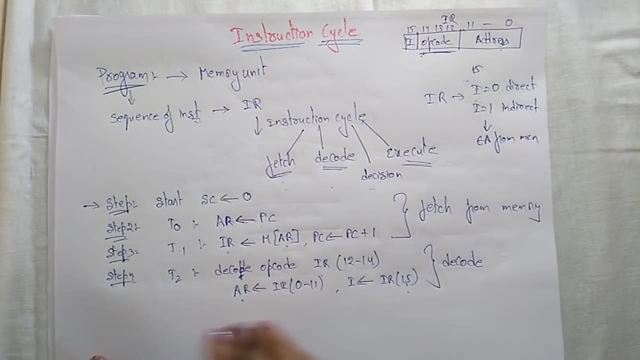 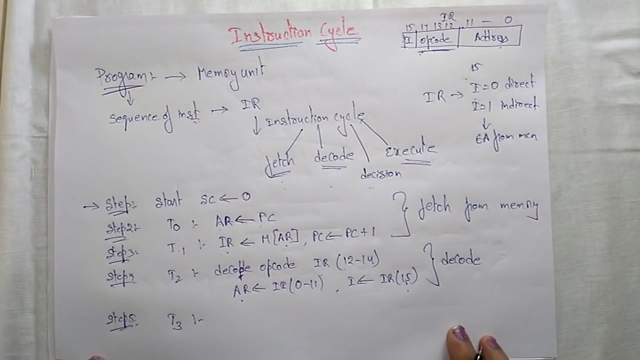 therefore, now you have to perform the direct addressing. so this is the decode section. so, whatever the data that is fetched from memory, that will be decoded. now coming to the step 5. so after that uh, decode, we have to execute the. we have to execute the decoded instruction. so before execution, we have to check. 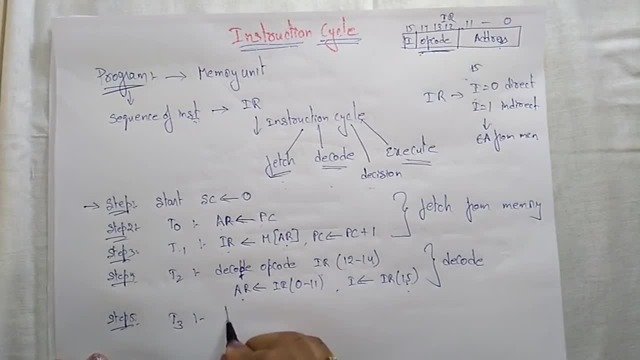 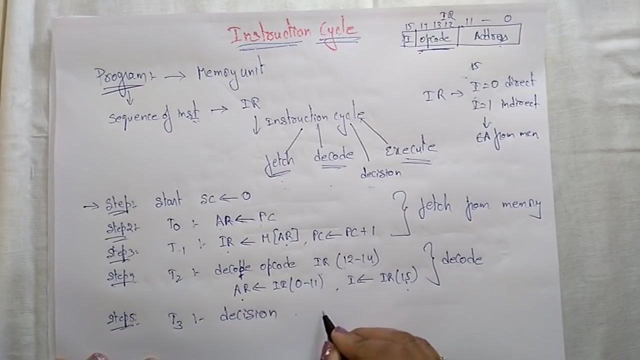 whether it is a direct address or indirect address decision taken place in this timing signal. so if it is actually the instruction register, the whatever the data instruction that we will taken from memory will be of three types. so the instruction may be a memory reference instruction register, reference instruction. 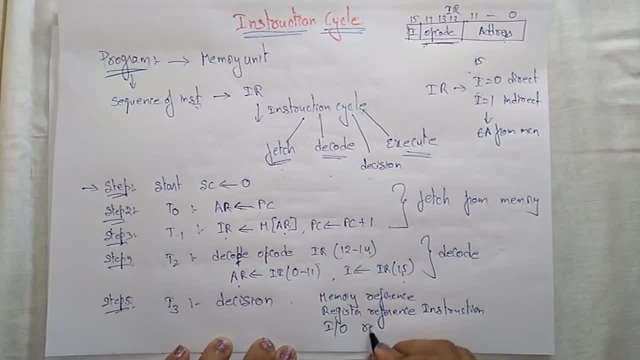 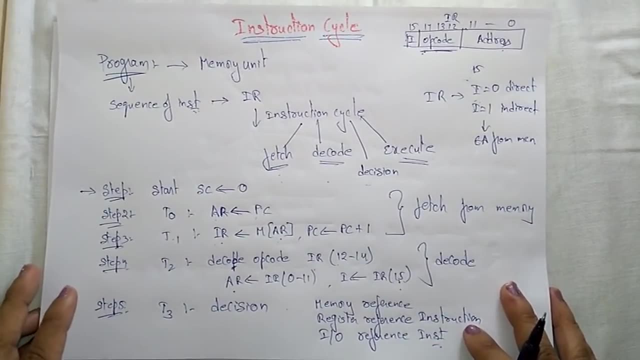 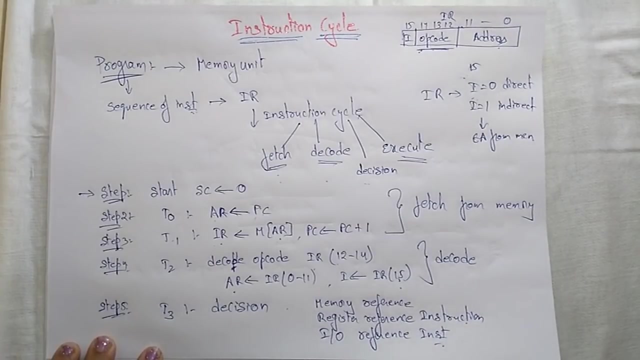 or input-output reference instruction. so the instruction, whatever we are getting from memory may be a memory reference instruction, register reference instruction or i o reference instruction. so these uh instructions will be means we have to uh. the d7 bit will decide the type of instruction: whether it is a memory. 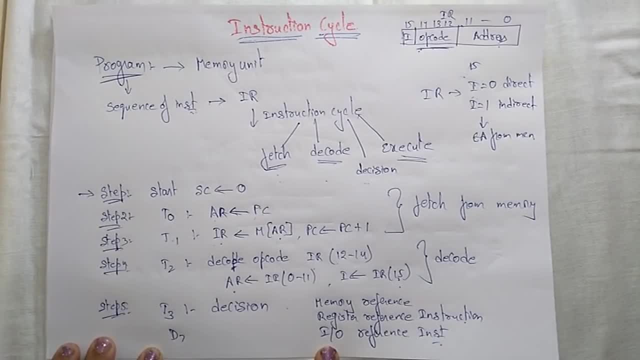 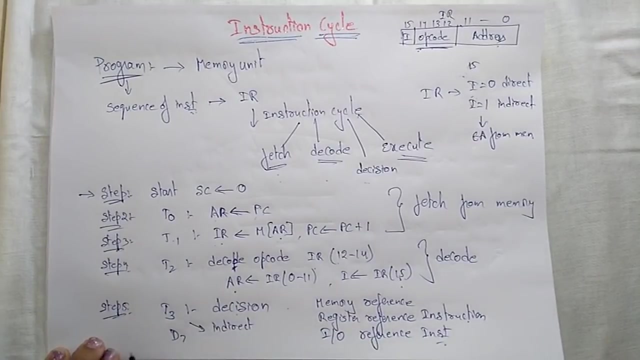 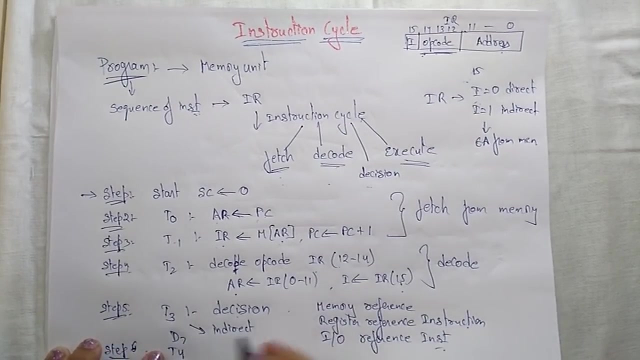 reference, register reference or i o reference. so this everything will be seen in the flow chart. so during t3, if it is not a direct addressing means. if it is, if t3 is indirect, the execution will be taken at t4. if it is direct, the execution will be directly taking place at t3 cycle itself. 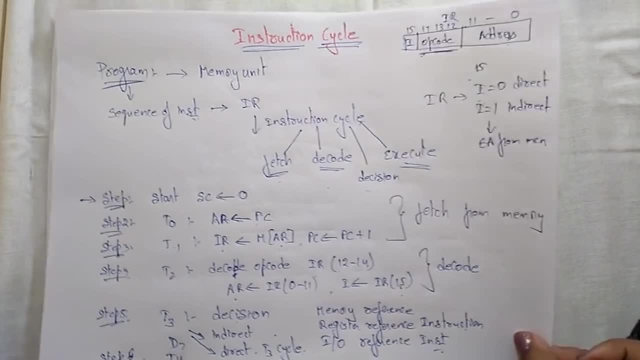 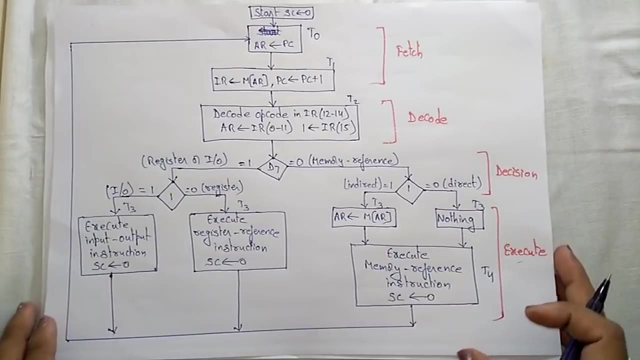 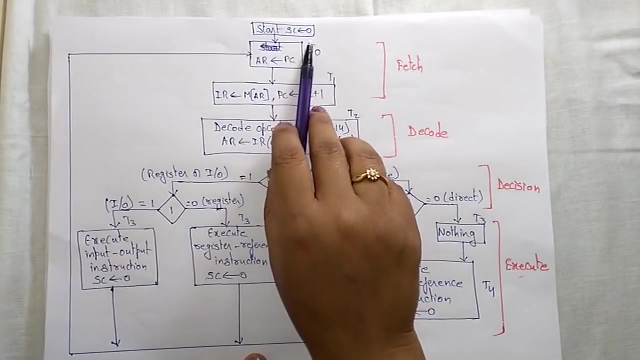 so let us see the flowchart of this instruction cycle. so this is the flowchart of the instruction cycle. here you have seen that start sequence counted to zero, so we have to start this. uh instruction, fetch, decode and execute. execute with the starting step. that is the sequence. 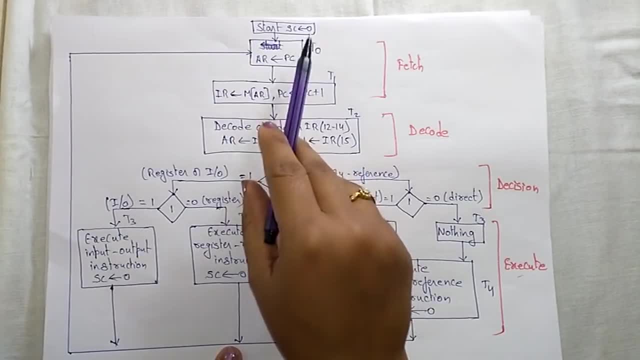 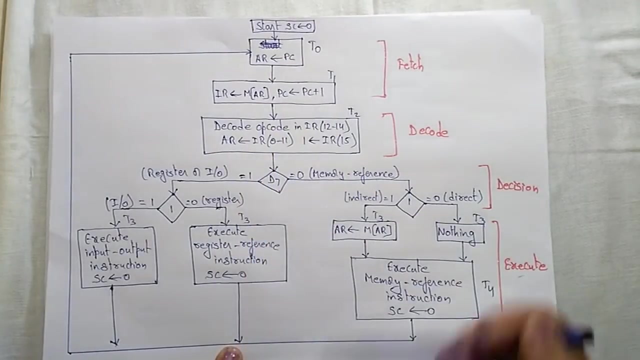 counter has to be cleared to zero. so whenever it is cleared to zero the pulse will start from t naught. so during t naught the program counter will be placed in the address register and after t1, pulse means uh, the pulse will be. timing signals will be incremented one by one. so 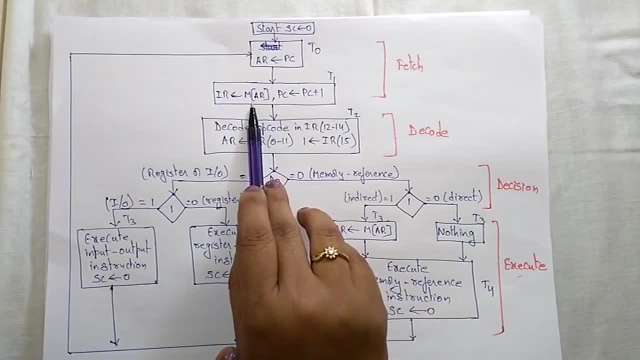 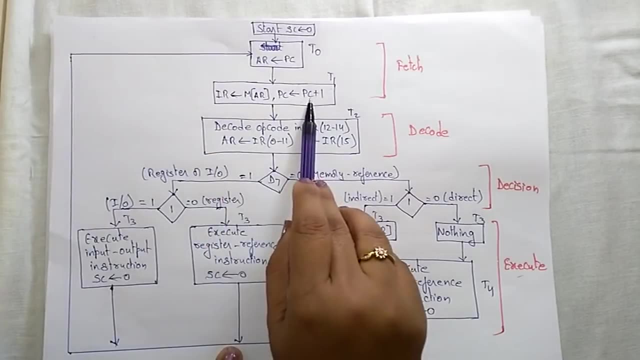 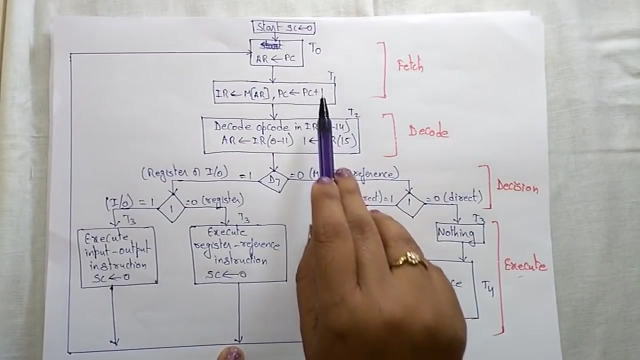 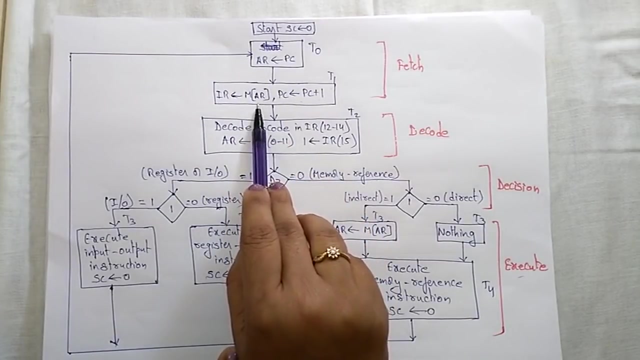 during t1. the program count uh. the memory address register. the address register uh memory reference will be placed in the instruction register. after that the program counter has to be incremented by one, so means it is going moving to the next memory location that will be stored uh in address register. so here the memory will be uh. 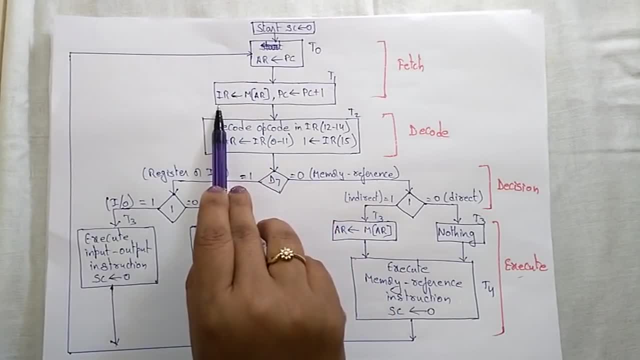 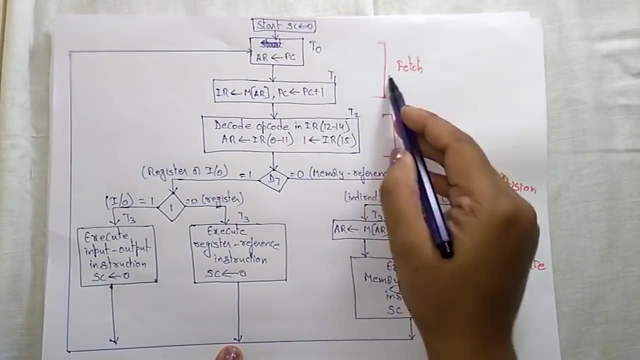 whatever the operation that has to be performed, that will be moved to the instruction register. so this, everything will be done in the fetch cycle. now coming to the decode: after fetching the data from memory, so memory- you have to fetch the memory from memory. so, after fetching the data from memory, 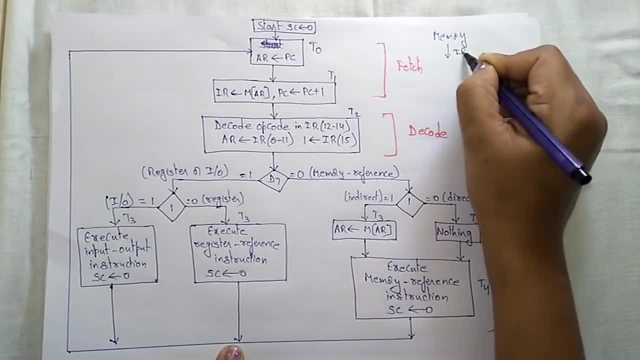 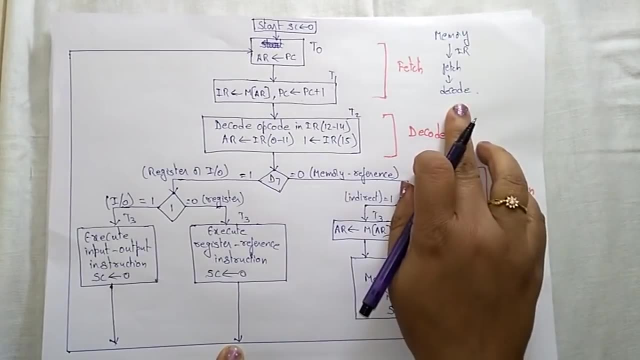 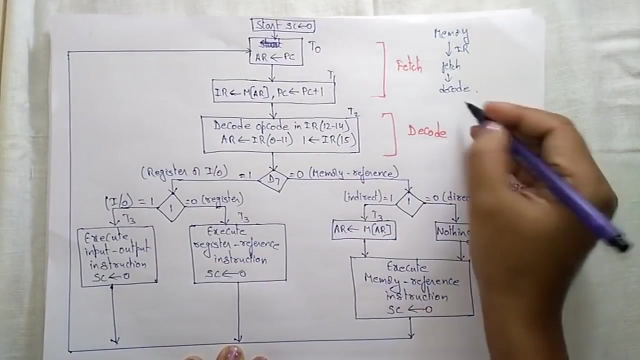 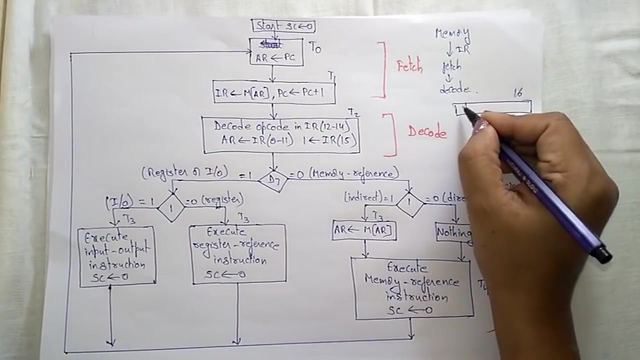 after fetching the data from memory. so memory, you have to fetch the instruction. after fetching, you have to be decode. so what we have to be decode. so whatever the data that is present in the opcode operation has to be performed. so i already said so, instruction register is of 16-bit register, so here the 15, 15th bit. 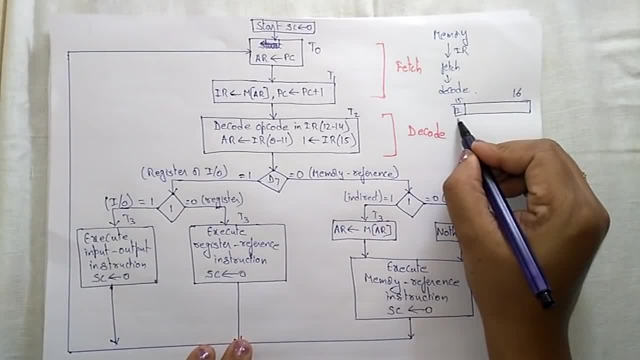 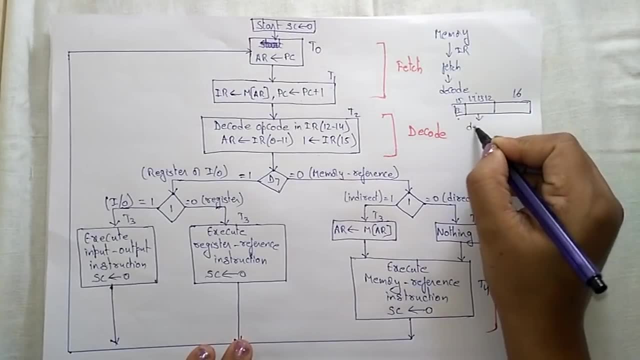 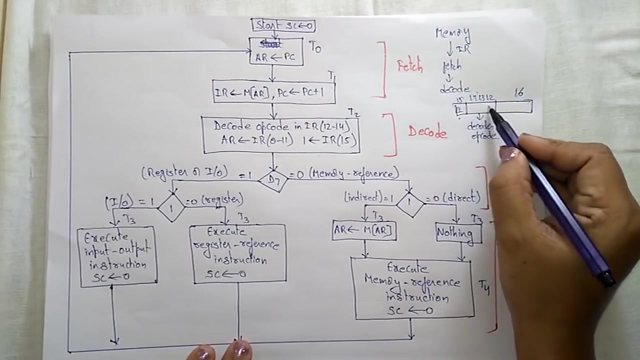 indicates the i, so it decides whether it is a direct address or indirect address, and 14-bit 13-, 12 it indicates the opcode. the decoded opercode. operation has to be performed will be placed in 14, 13, 12 and from 11 to 0 address will be stored. 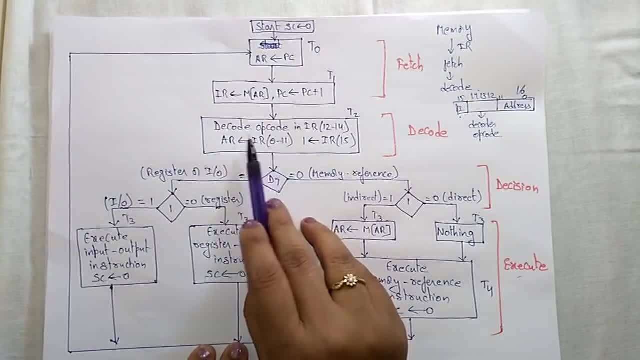 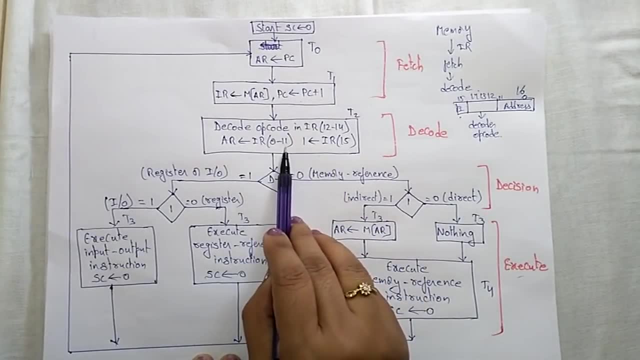 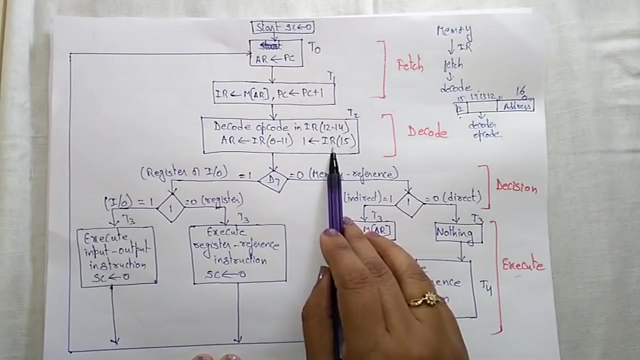 so here: uh opcode, uh decode. opcode means the operation has to be performed. will be placed in instruction, registered 12 to 14 and uh zero to 11 is the address will be placed in the address register and the 15th bit of i in the instruction. 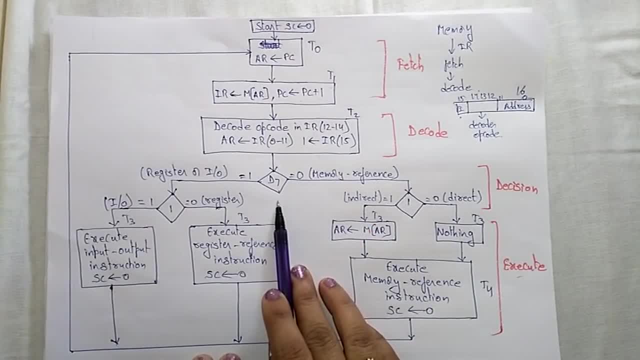 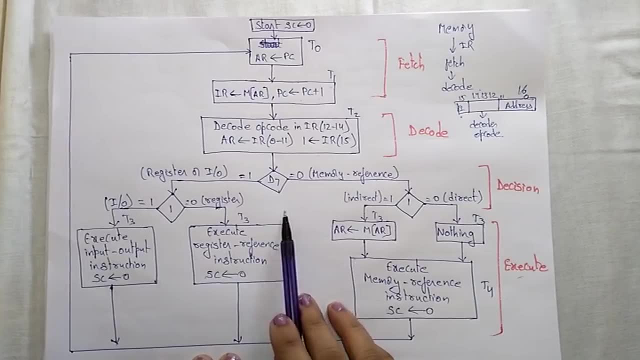 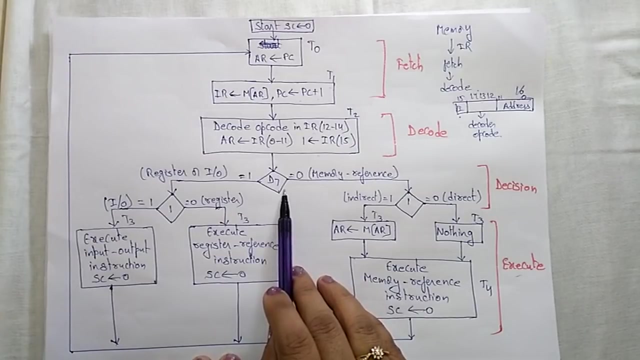 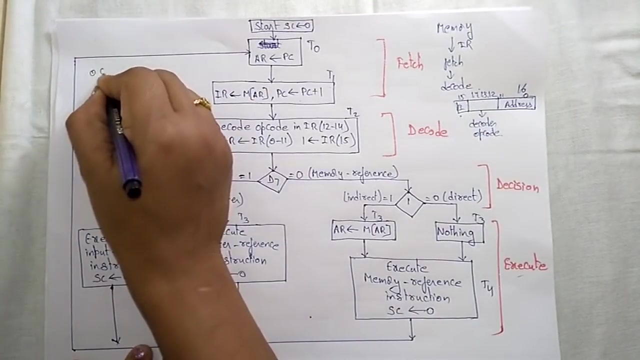 register will be placed in i. so now, coming to the after decoding, we have to execute the program. so before executing the program, we have to check whether the data is direct or indirect. so coming to the d7, so actually this 14, 13, 12 is from it's a 3 bit, 0 to 1, 1, 1 will be there. so this: 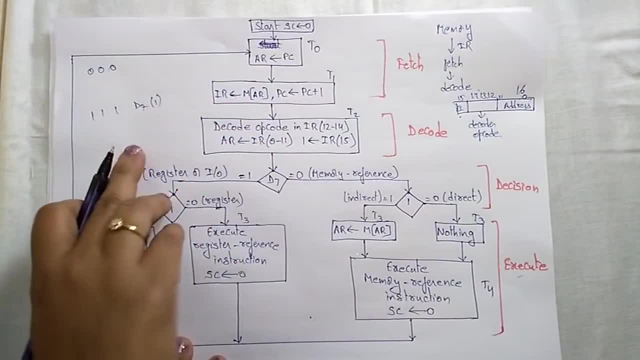 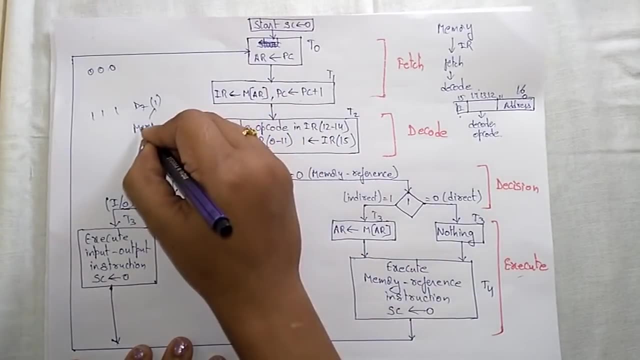 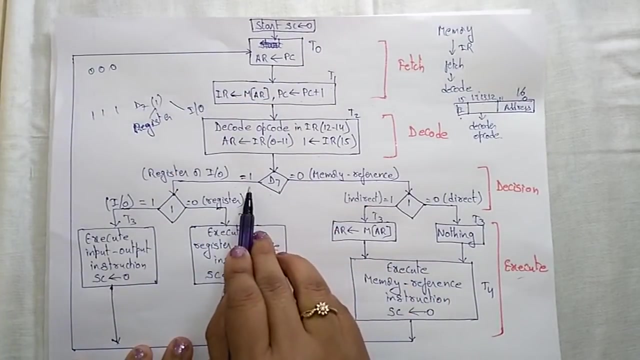 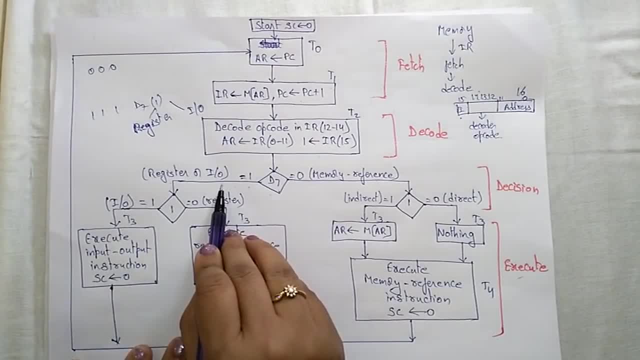 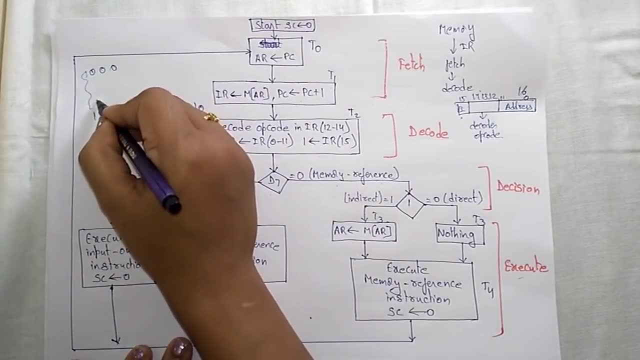 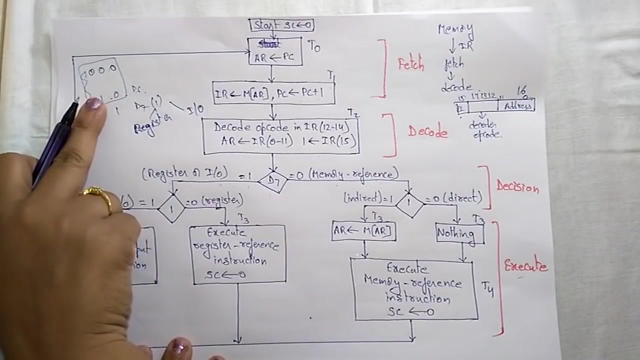 a register reference or io reference instruction. whether it is 0, it compulsory. it should be a memory reference. 0 means any one of this from up to here, from 0: 0 to 1. 1. 0 means d6. these are all allocated to memory reference and the last one is the whether it is a register. 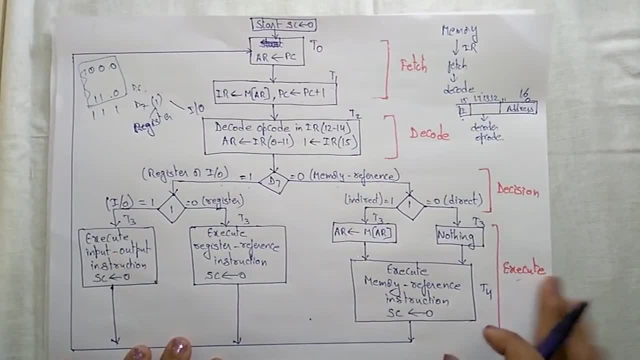 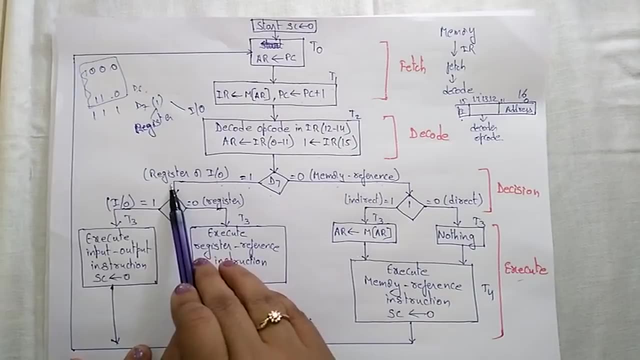 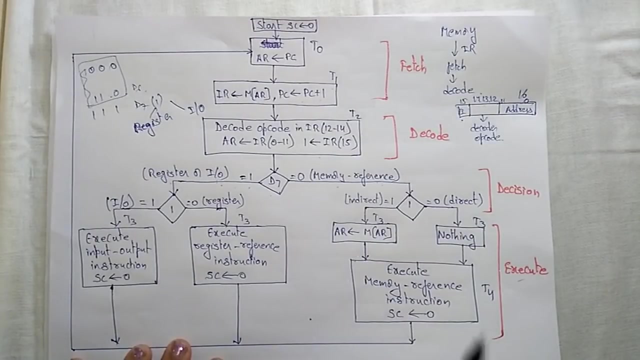 reference or io reference. so i already said the instruction is of three types: memory reference, io reference, register reference. first we have to decide which instruction is it. is it a memory reference, io reference or register reference? we have to decide. so this is the decision place. so suppose if you 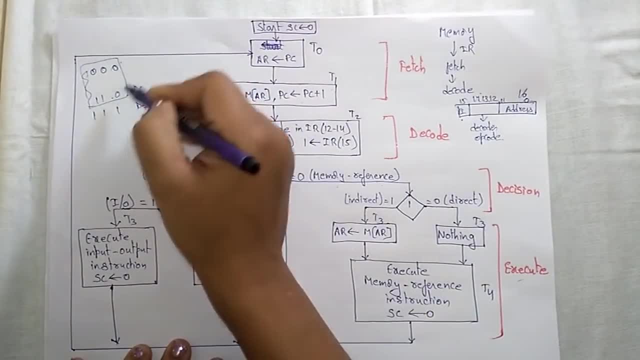 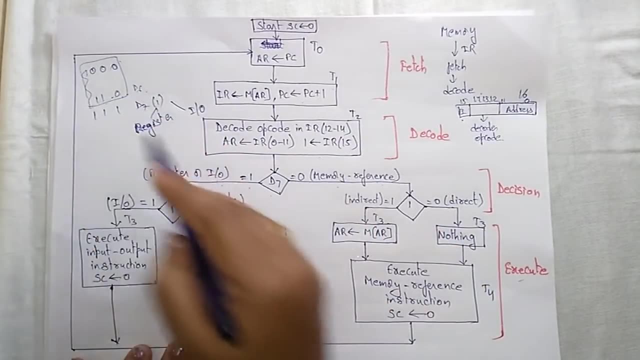 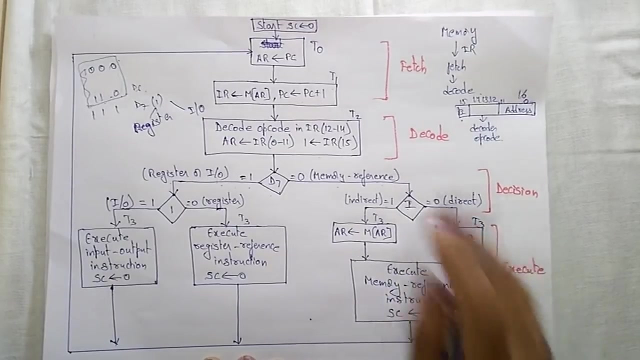 take it is a memory reference means from 0 to 1, 1, 0. so okay, the instruction is a memory memory reference. it is in between these instructions. so if the- I now check I this I is direct or indirect. suppose it is direct. direct means, suppose memory. 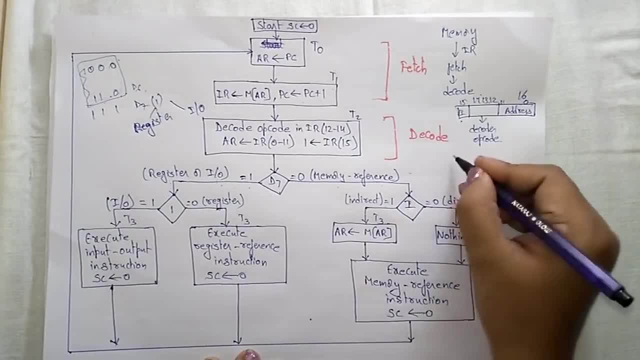 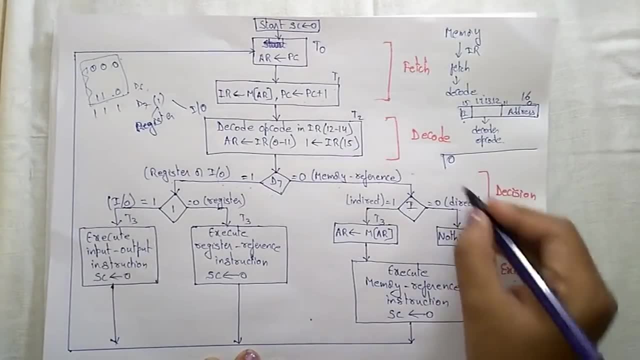 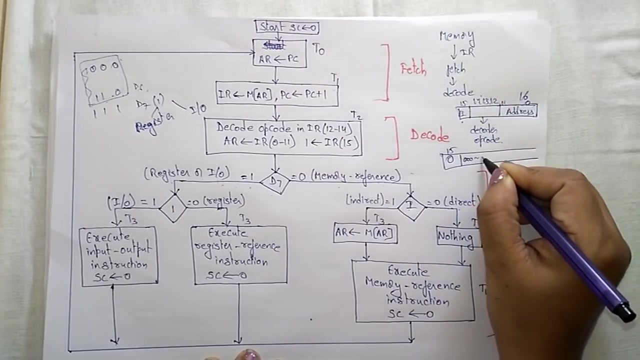 reference: direct means. direct means 0, 0, 0. this is 15th bit. it is 0 and it should be in between 0, 0 to 1, 1, 0, anything 14, 13, 12. this bit be anything and the remaining. 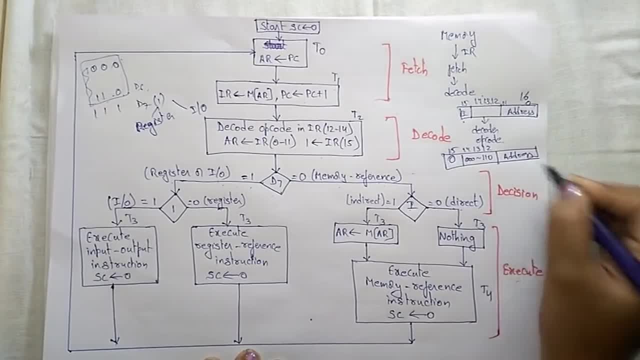 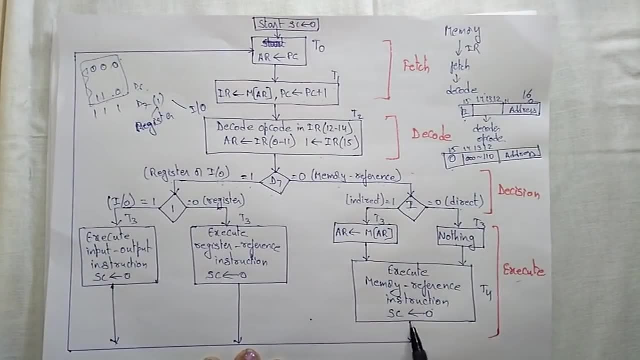 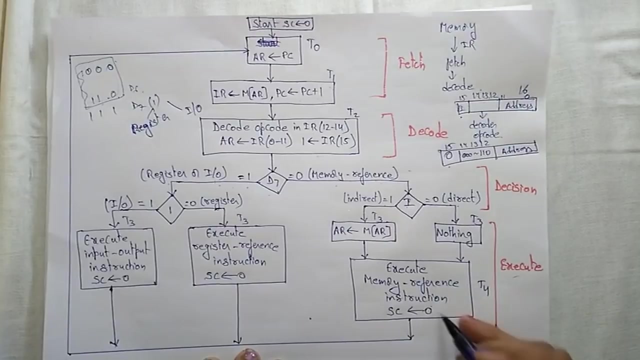 is the address. so if it is 0, nothing we have to be do directly. you have to execute the memory instruction and you make the sequence counter to clear to 0, because you execute the instruction after execution, executing the instruction again, the cycle will starts from 0. 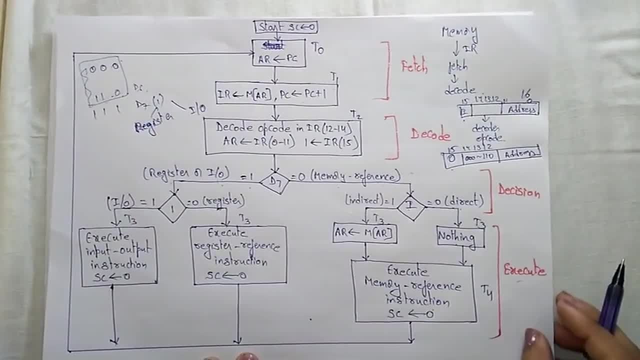 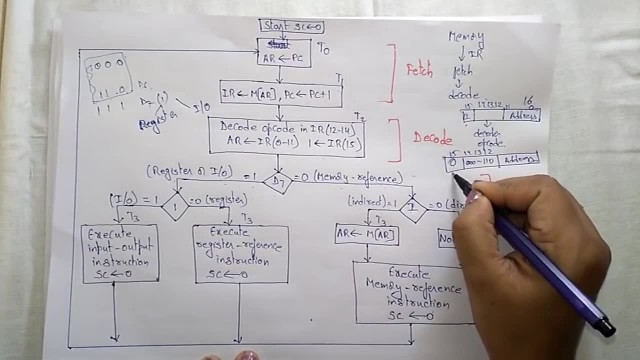 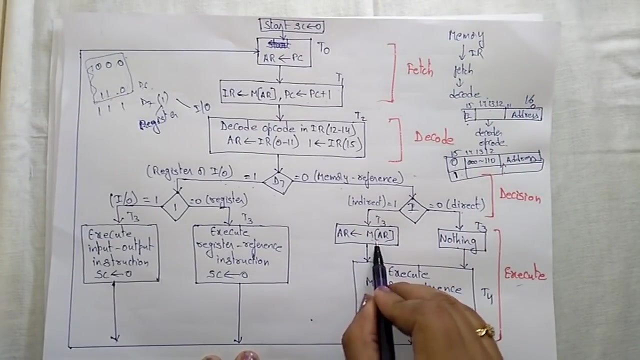 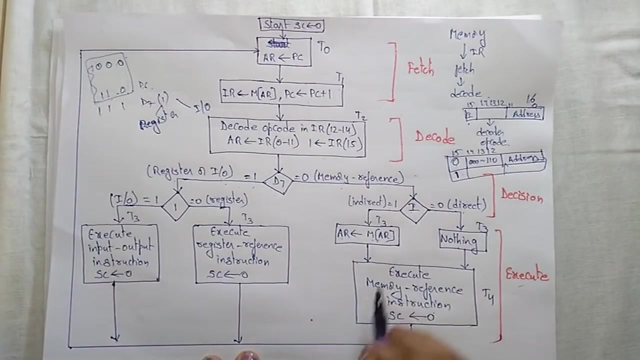 0, again the cycle will starts from 0. suppose it is 1. suppose this is 1. means this is 1. so what we have to do? if it is 1, we have to be convert. means you have to take the effective address register in AR. then you have to execute the memory instruction. means you have to take 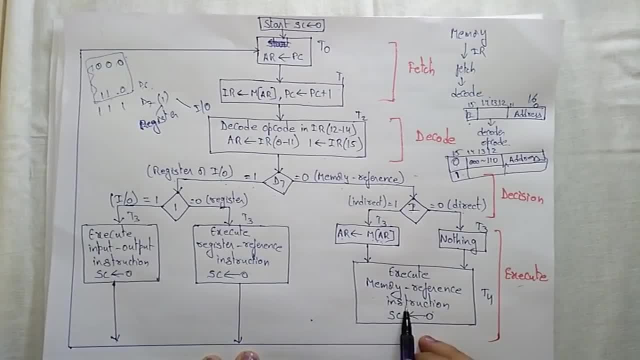 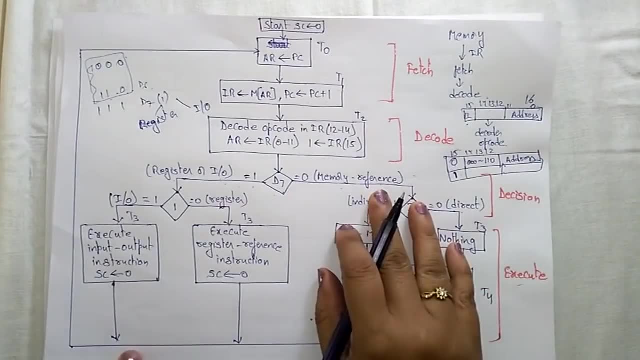 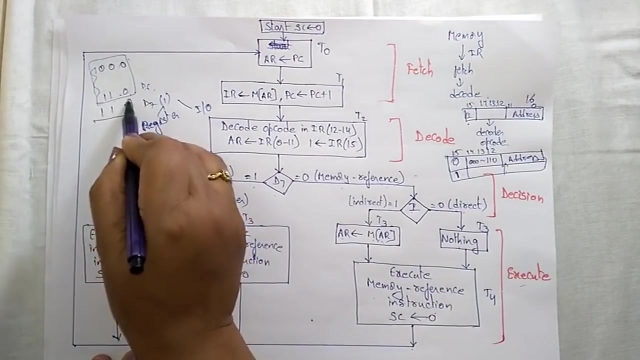 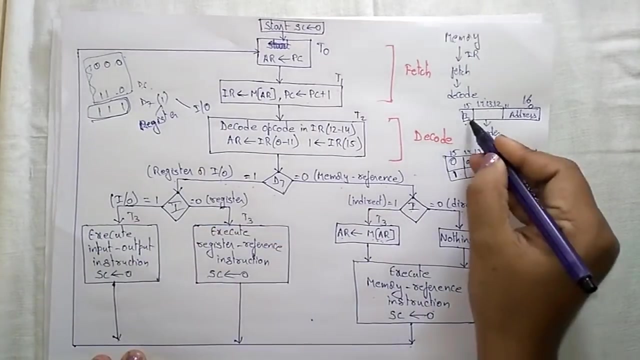 the data from effective address register and then you have to execute the memory reference instruction and make the sequence counter to 0. so this is about memory reference. now coming to the register reference or IO reference. suppose D7 is 1 means this is the last bit, D7 is 1. if D7 is 1, suppose the I, the last bit is the last bit, is 0, means 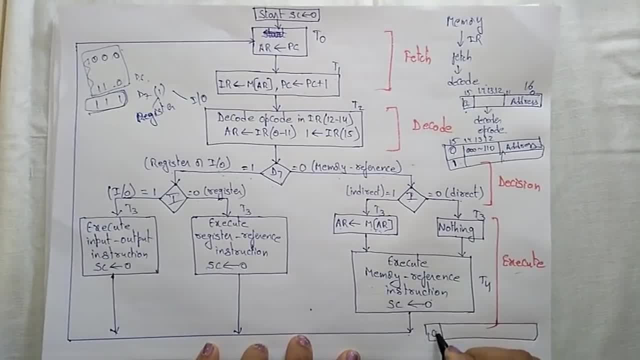 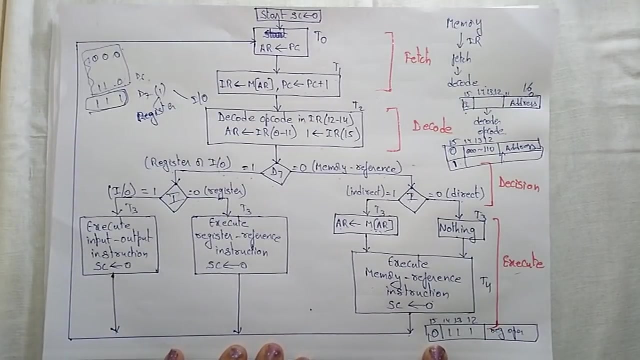 what if the last bit is 0 means D7 is 1.. 15th bit is 0 and 14, 13, 12 or 1, 1, 1 and the remaining or the register operations. okay, if it is like this, the instruction is like this, then you have to execute register reference. 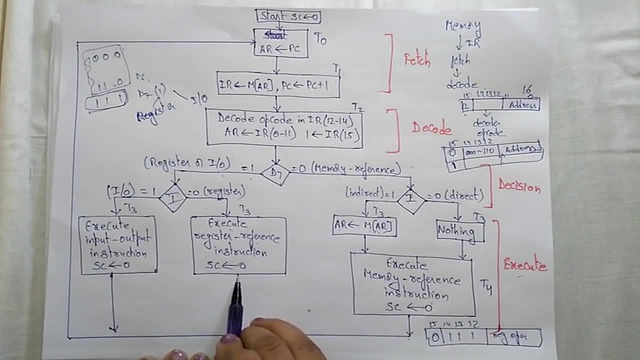 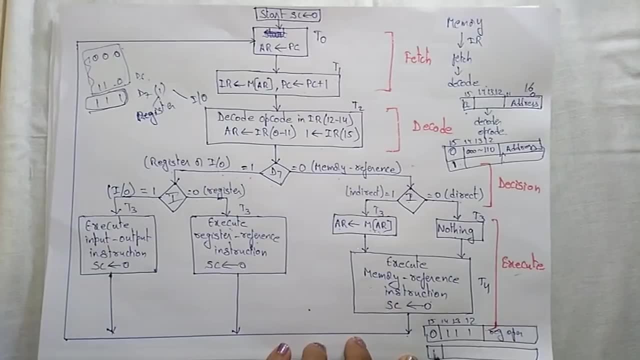 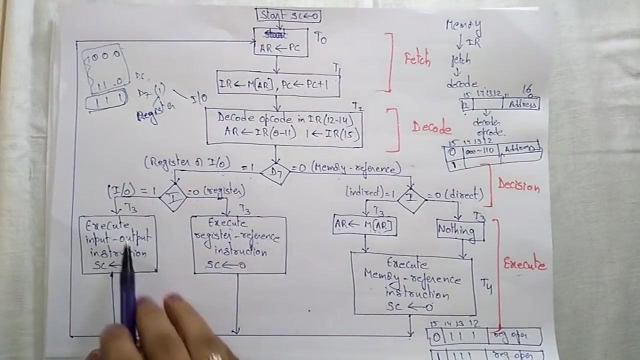 instruction and make sequence counter to 0. suppose if it is the I is 1. suppose the I is 1 and then opcode is 0.. 111 and the register operations. then you have to be execute input output instructions and make sequence counter to 0. again you have to start the next cycle. so this is how the 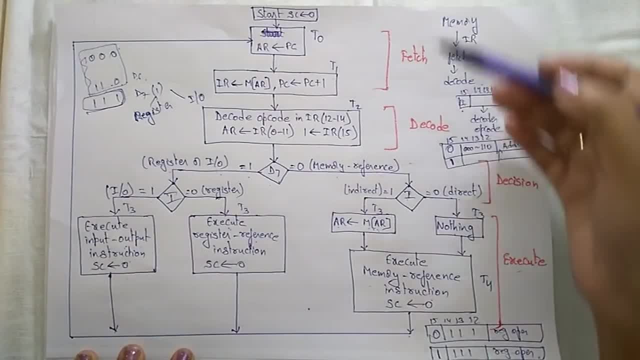 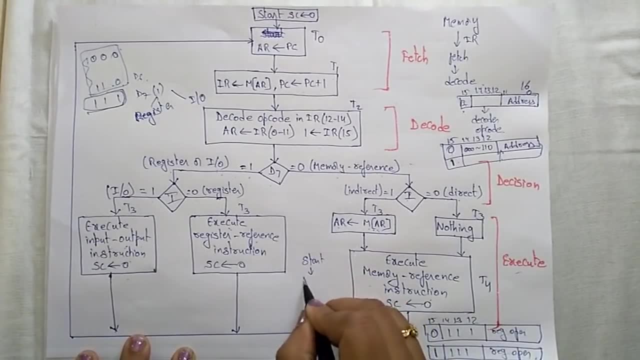 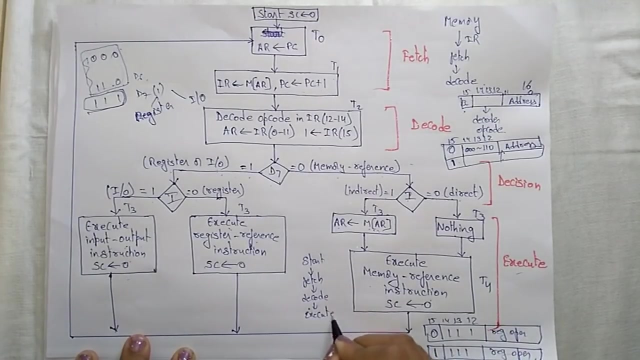 instruction will be executed internally. so this is the instruction cycle. so 1: start start fetch decode 1., 2., 3., 4., 5., 6., 7., 8., 9., 10., 11.. 12., 13., 14., 15., 16., 17., 18., 19., 20., 21., 22., 23., 24., 25., 26., 27., 28.. 29. 30., 31., 32., 33., 34., 35., 36., 37., 38., 39., 40., 41., 42., 42., 43., 44.. 44., 45., 46., 46., 47., 48., 49., 50., 51., 52., 52., 53., 53., 54., 53., 54., 55.. 56. 56..